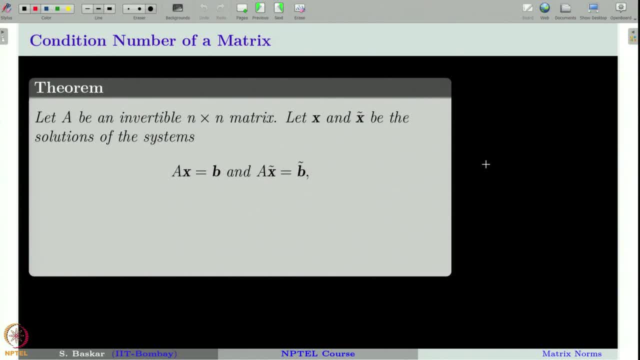 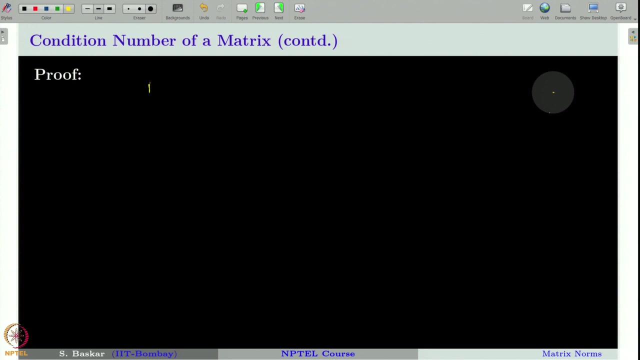 x. So let us denote this solution from the perturbed system A x equal to b tilde as x tilde. In linear systems we can write A x minus A x tilde is equal to b minus b tilde From: 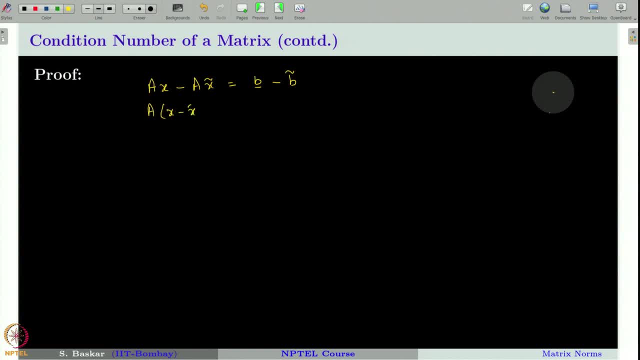 there we can write A into x minus x tilde is equal to b minus b tilde, Since A is invertible. therefore, we can write x, x minus x tilde is equal to A inverse into b minus b tilde. Now let us take norm on. 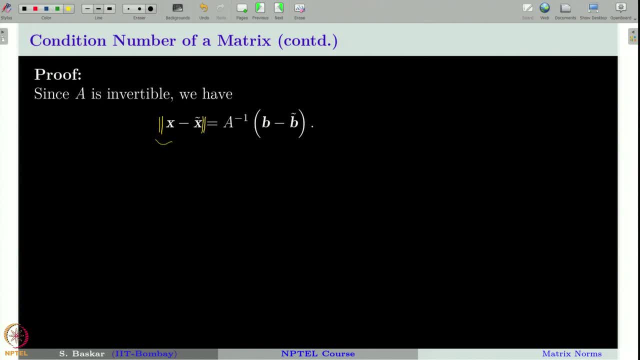 both sides. Remember, this is the vector norm and this is also the vector norm right Now. you recall from our last lecture we have proved an important property: A is actually an important property for the subordinate matrix norm, which says that A 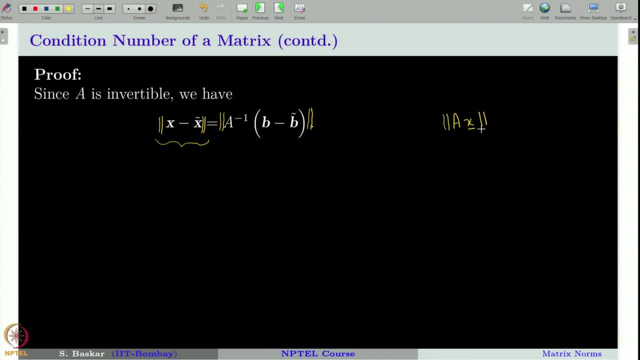 x, which is a vector, and you take the vector norm on that, Then you can write this as less than or equal to norm A, which is the subordinate matrix norm times norm x. right, We have proved this inequality in the last class. Now you see, you can just imagine this, as A is equal. 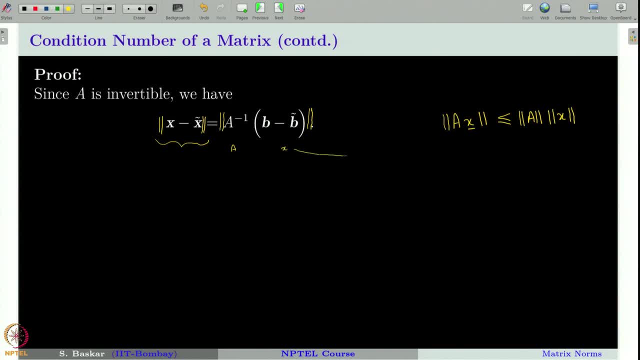 a and this as x, and you can apply this inequality to get norm x minus x tilde is less than or equal to norm a inverse, because you have inverse here into norm b minus b tilde. that is the vector here. right Now we have this in one hand, right see, remember we have to prove something. 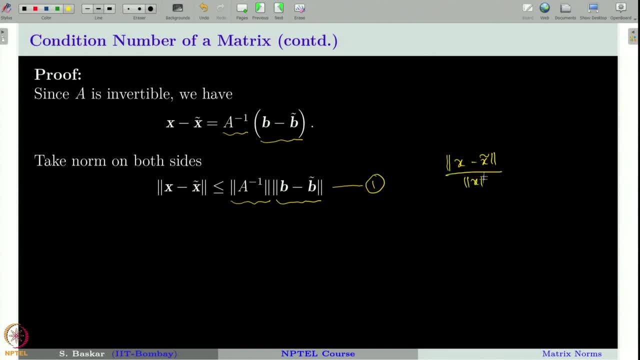 for the relative error. So we have norm x minus x tilde. now we have to divide both sides by norm x. that is what we have to do here now. Now you remember, this is less than equal to norm a into norm a inverse, into b minus b tilde divided by b right. but here we have 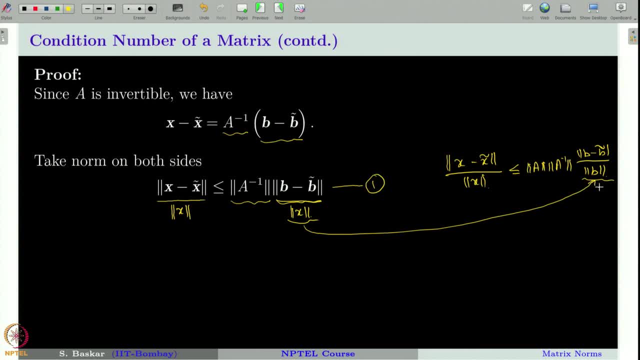 x, but we want b tilde here, right. So we have to somehow dominate this x by b here. how will you do that? Well, let us go back to our original system: a. x equal to b And take norm on both sides, norm on both sides. you will get norm. b is equal to norm. 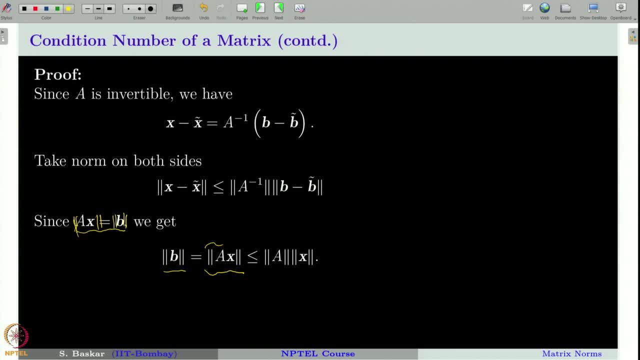 a x. Now, whenever you see this, immediately our property should come in your mind and you can write it as norm a. x is less than or equal to the matrix norm a into vector norm x. Right, that will immediately tell you that 1 by norm x. what I am doing? I am just taking. 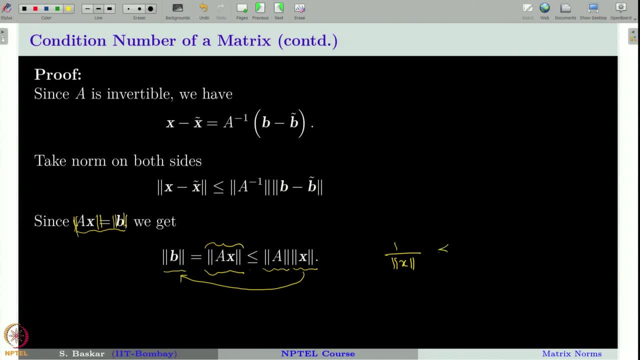 this to the left hand side, and that is less than or equal to norm a, and this I am bringing to the right hand side, and that will come as norm B. So this is precisely what we were intend to do: this ло To norm a. 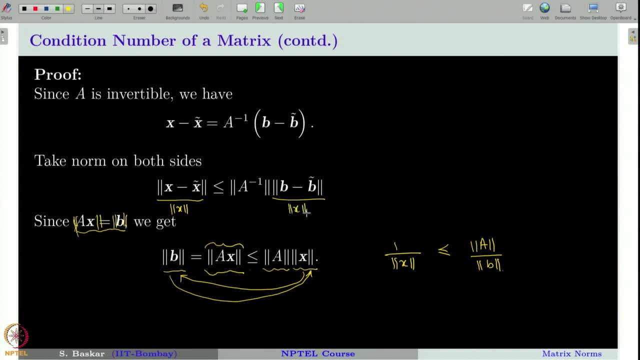 This is norm b x negativity. The porta ra n divided by norm x was what we had in the previous inequality. Now this part is less than or equal to norm a divided by norm b. Therefore, you can write: this is less than or equal to. 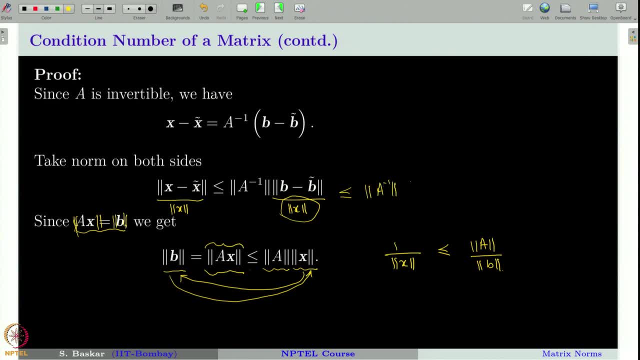 norm a inverse into norm b minus b tilde. these are there already Now. instead of 1 by norm x, we will put this. that is why I have this less than or equal to sign. here I have norm a divided by norm b. that gives me precisely what we want. I will repeat once again what 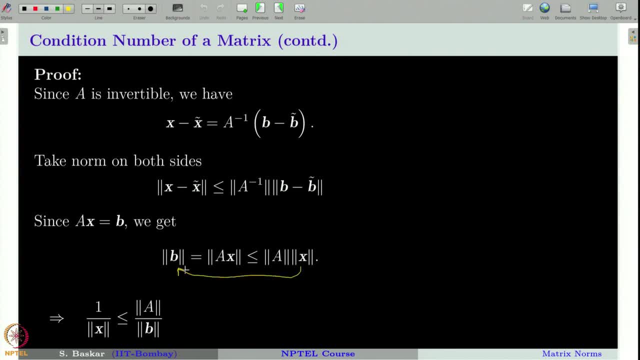 we are doing is we are taking this to the left hand side and b to the right hand side and writing this inequality from there. We are getting what we want by putting this inequality into this. So remember: first we have divided by norm x on both sides and then we put this inequality here to get this. and this is precisely. 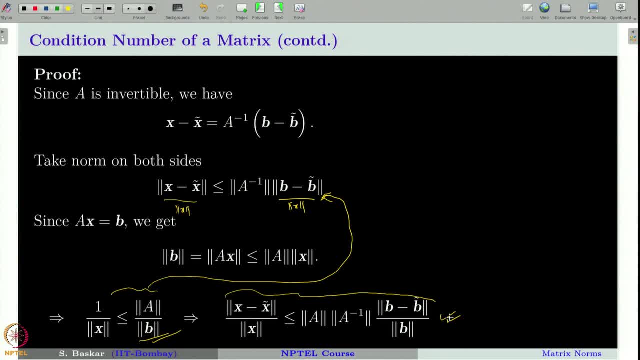 what we want to show. So this is a easy proof, but the result is very important, which tells us that the relative error in the approximate solution when compared to the exact solution is amplified by this factor with respect to the relative error in b tilde when compared to b. that is the 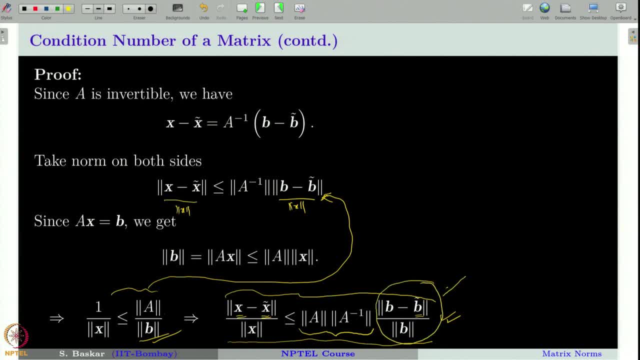 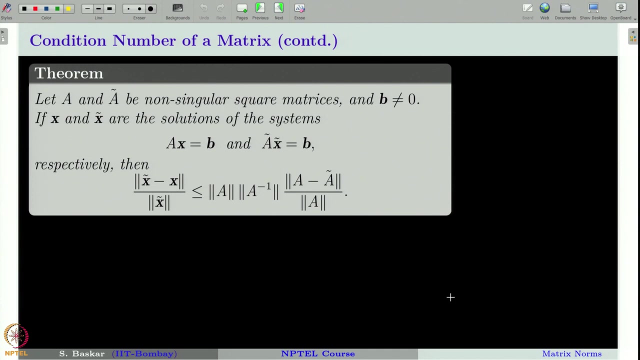 error you have committed in your input data. So remember, this theorem is only considering the error in the right hand side vector, whereas matrix is taken exactly. but in practical situations we will have error even in the coefficient matrix. So let us see how the estimate for the relative error in x tilde. 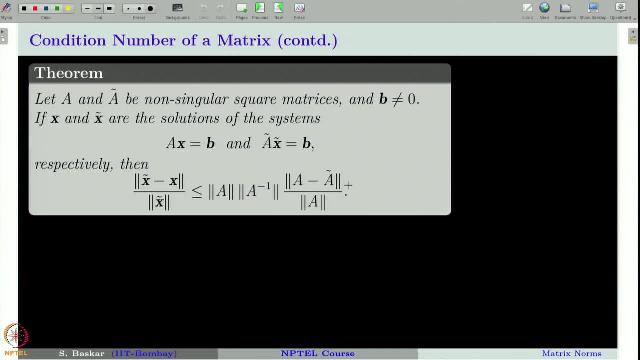 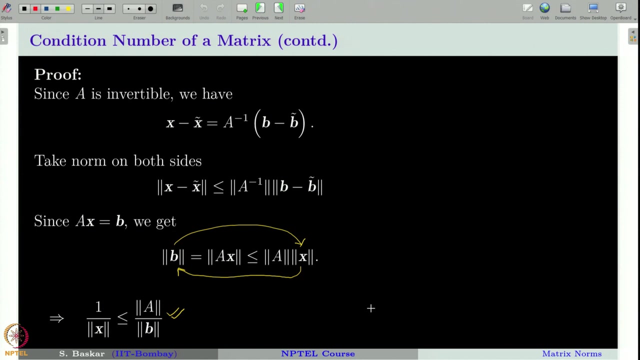 will look like when compared to the relative error in the coefficient matrix, and that is given by this inequality. Here also, you can see that this expression is coming as the factor here. in the previous one also, the same expression was there, So that shows. 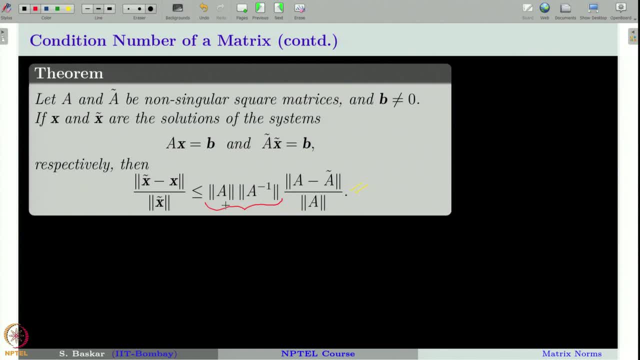 that this quantity, that is, norm A into norm A inverse, is very important in understanding the relative error in the coefficient matrix. So let us see how the estimate for the relative error in x tilde will look like when compared to the relative error in x tilde. So let us 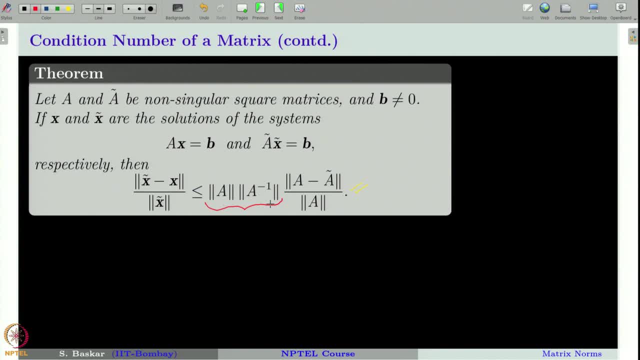 see how the estimate for the relative error in x tilde will look like when compared to the relative error in x tilde. So let us see how the estimate for the relative error in the approximate solution of your linear system when compared to the exact solution. 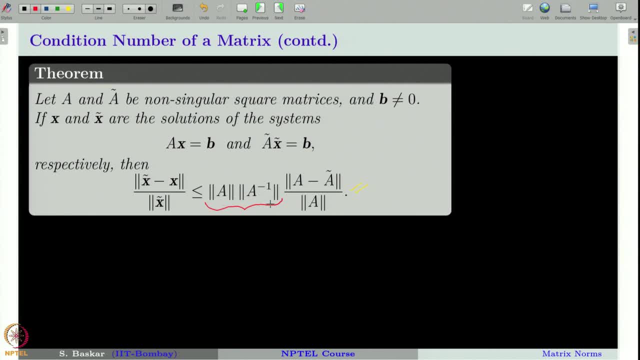 So now, how to prove this theorem. well, it is not very difficult. we can prove it with a little mathematical manipulations. Let me quickly tell you. you can fill up the gaps. you start with this: A x minus A tilde, x, tilde. This is how we have started our proof in the last theorem also. but now you see. 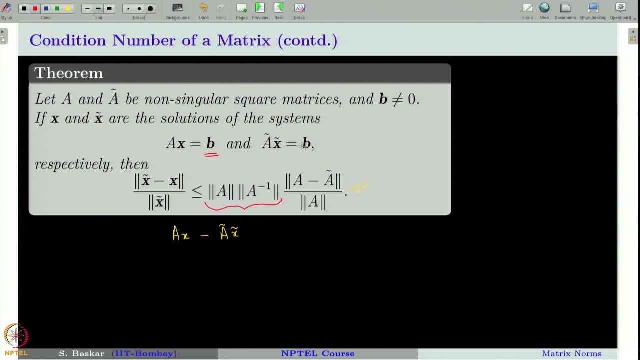 you do not have any error in your right hand side vector. You are now considering in this theorem that the right hand side vector is exact, but you have error only in the coefficient matrix. In the previous case it was the other way round, In fact, in practical situations. 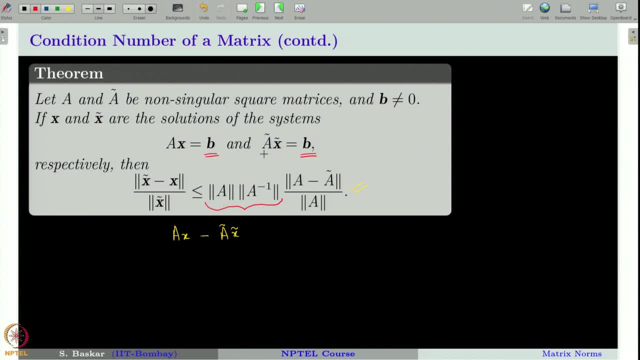 we have error in both these inputs but for the sake of simplicity, we are considering these two cases separately and getting the inequalities. You can also combine and get any inequality, but that you can do it once you understand these two steps. Therefore, I am only doing these two steps separately. Let us start with this since the right hand. 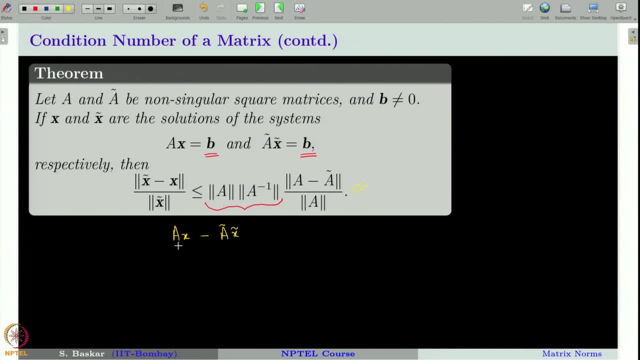 side vector is same, you will have a x minus a tilde, x tilde equal to 0.. Now what you do is you add and subtract a x tilde, that is, a x which is already there, minus a x tilde which you newly insert into this equation. 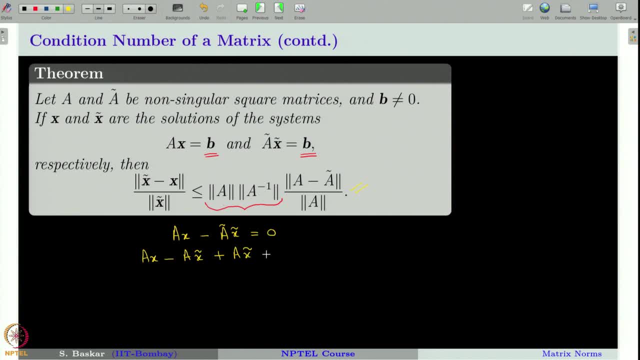 Then you add the same quantity and then you take a tilde- x tilde, which is already there, equal to 0. That can be written as a into x minus x tilde, equal to a minus a tilde. There is a minus sign here because you are taking to the other side and x tilde. That implies, since a is. 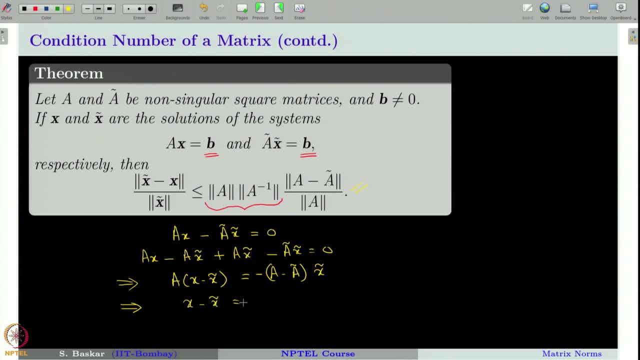 invertible x minus x tilde is equal to minus a inverse into a minus a tilde. So this is a into a minus a tilde, x tilde. Now you take norm on both sides. The remaining part of the proof will go more or less in a similar way as we did in the previous theorem. I leave. 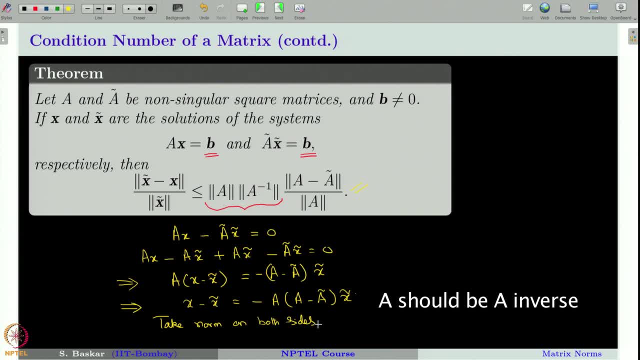 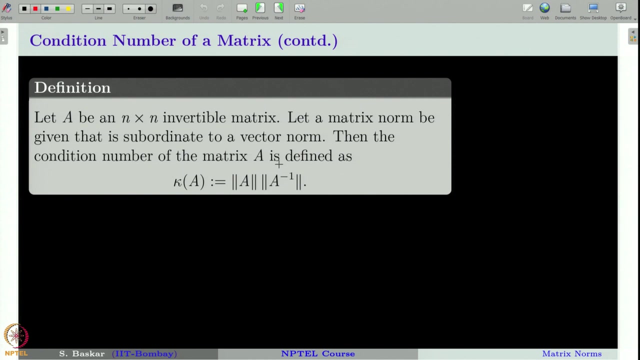 it to you as an exercise to complete this. Now you see the important point. as I mentioned, this quantity seems to be very important in quantifying, at least as an upper bound for the relative error. Therefore, we will take this quantity and give the name as condition number of the matrix A. So we will define. 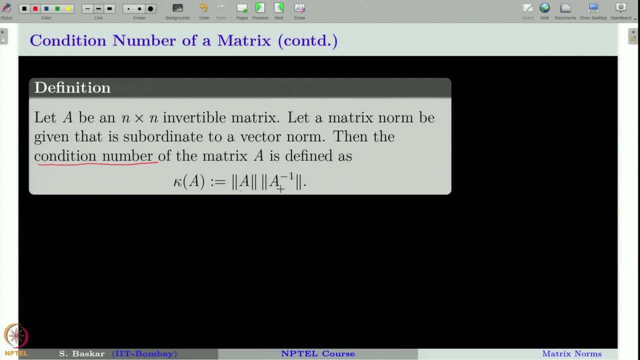 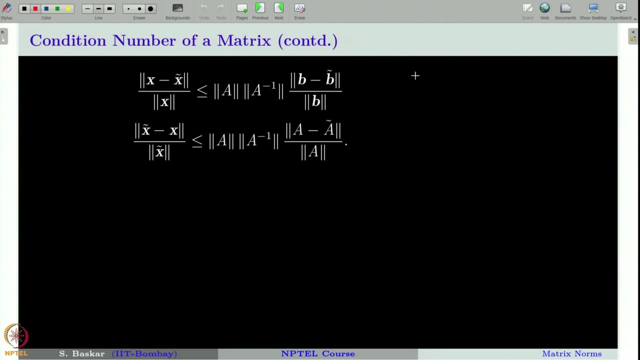 norm A into norm a. Norm A inverse as the condition number of a given n cross n invertible matrix. We generally use the notation kappa of A for this. So let me summarize: when we have the error only on the right hand side vector, that is. 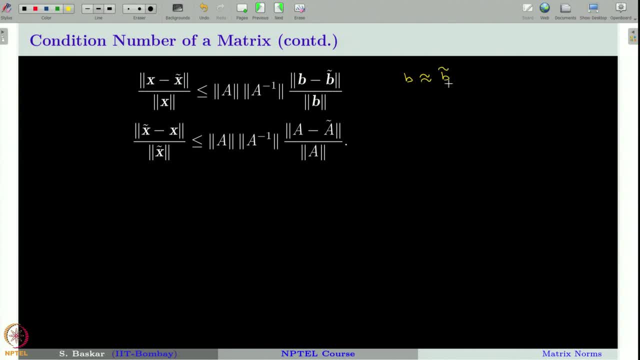 B is taken as B tilde with some error, Then the relative error in the corresponding solution of the linear system will have such an estimate. and similarly, if you have the error in the coefficient matrix, that is, instead of A, if you take an approximation to A, which is 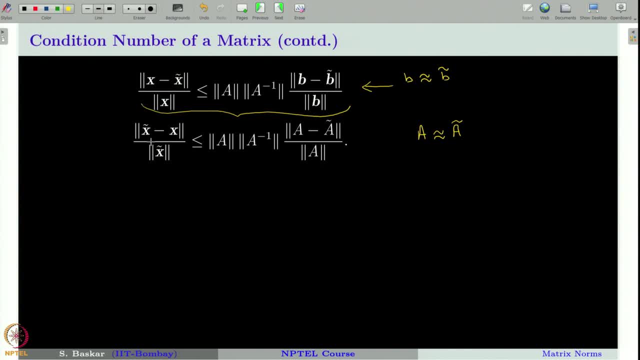 denoted by A tilde, Then the corresponding relative error in x tilde when compared to x is given by this estimate. In both the case the amplification factor is nothing but the condition number kappa of A. Now you can see that if kappa of A is very small for a 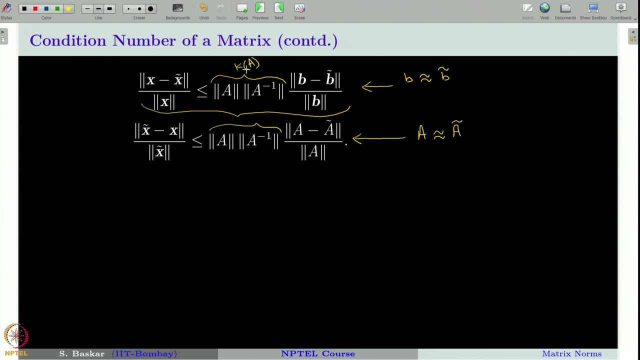 given matrix A, then if you assume that this relative error, equivalently this relative error, is very small, then the upper bound is going to be very small. Generally, it is fair to assume that this relative error in the input data is very small because that: 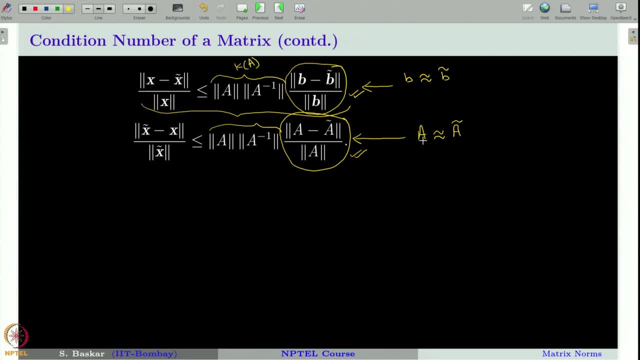 comes as most probably the rounding error on your computer, or it may be some small error that we may make somehow. Therefore, these relative errors may be assumed to be very small. Therefore, if the condition number of your coefficient matrix is very small, then 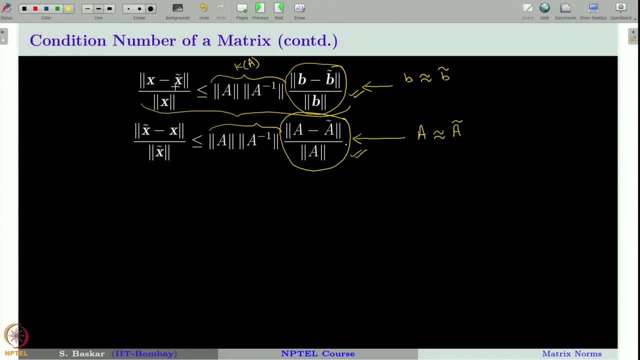 See, the relative error in the approximate solution will also be very small. On the other hand, if the condition number is very large, so large that this product becomes a big number- then what happens? It gives us a possibility that your relative error in the approximate 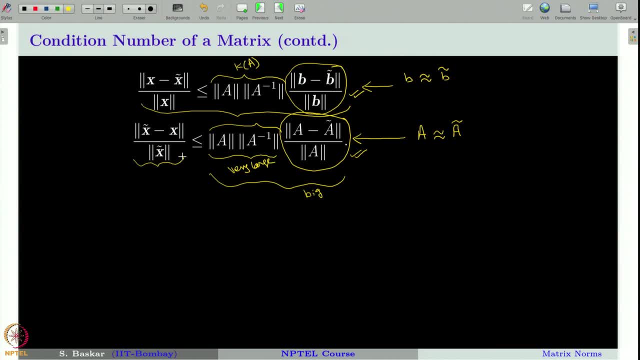 solution may also be very large. It will not tell that the relative error in the approximate solution will be surely large, but it gives us a possibility that this may be large. So that is a kind of caution that this condition number will give us. 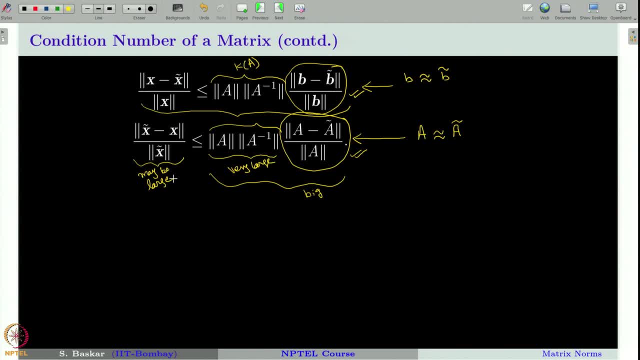 If your condition number is very large, then the computation of the solution of a linear system may be very small. It may be very sensitive to even small error in your input data. That is what the message we are getting through this analysis. Here we should note very importantly that the condition 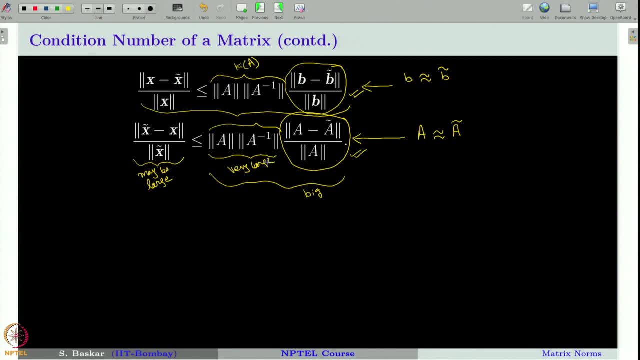 number of a matrix depends on the subordinate norm that we use. That is, we will first decide what vector norm we will be using, and from there we will have a subordinate norm corresponding to that vector norm. The condition number is then calculated with respect to that matrix. 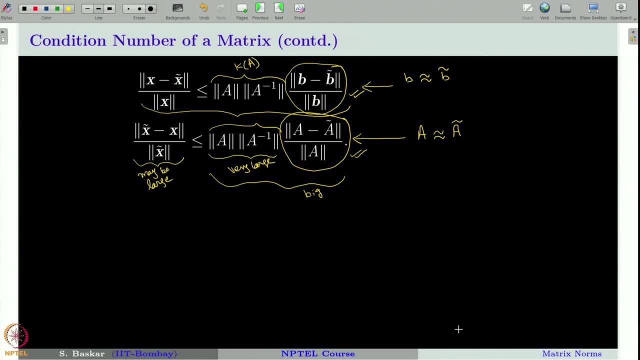 norm. Generally we will use infinite norm because that is the easiest norm, although it is not physically realistic, but it is easy to handle infinite norm rather than the L2 norm. So in all our analysis we will fix L infinity norm and compute the condition. 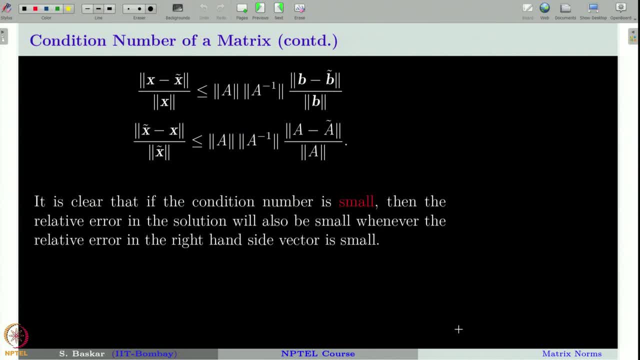 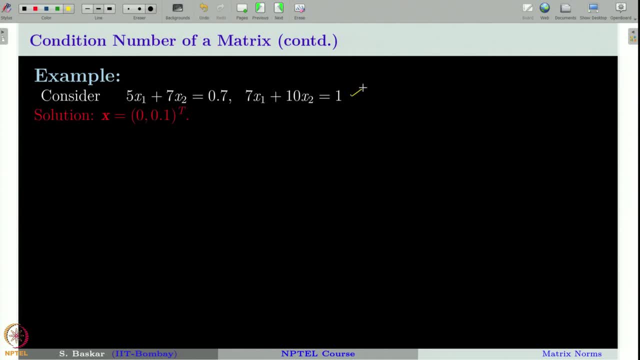 number of a given matrix. Let us take an example. Consider this system where the right hand side vector is 0.7 and 1.. The corresponding solution is 0.1.. Now what we will do is we will make a slight. 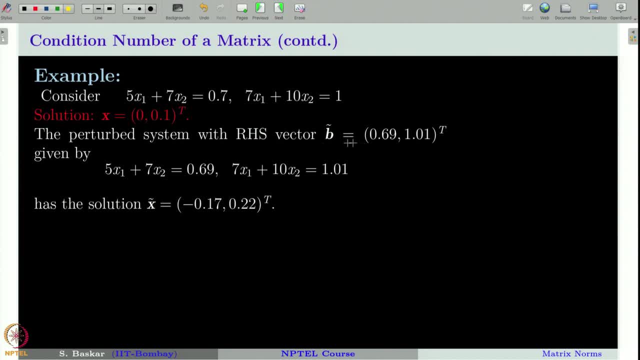 perturbation in the right hand side vector. thereby we will consider b tilde as our right hand side, which is given by 0.69- 1.01.. So this is slightly different from the right hand side vectors given here. So we have made a slight error in our right hand side. 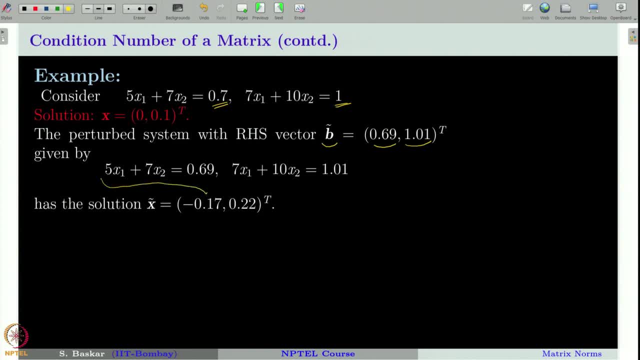 vector. Therefore, we are considering this system, but we are actually intended to solve this system and get this solution. but we are actually solving this system and therefore we are getting its solution, which is given by minus 0.17 and 0.22.. 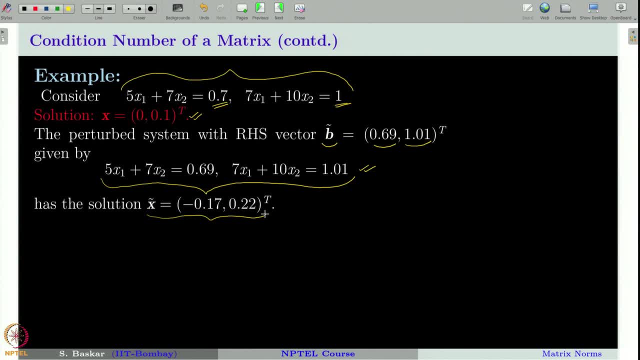 Let us compute the relative error in x tilde when compared to x and see how it looks like. Now, coming to precise computation like this, we have to choose one particular norm to do this computation. As I told you, it is very easy to handle L infinity norm. Therefore, I will take the. 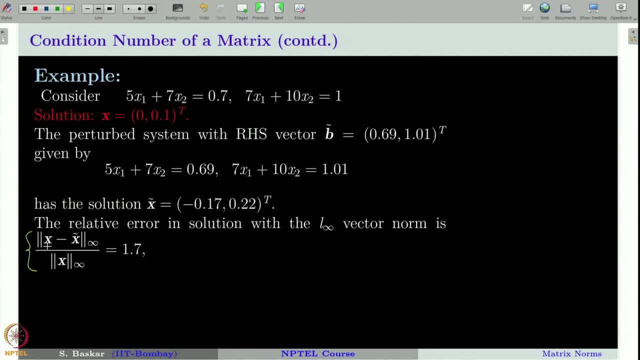 relative error in x tilde with respect to the infinite norm. Remember, infinite norm of a vector is defined as maximum of the components of the vector, its absolute value. So this is how it comes Now: if you take norm x minus x tilde, infinity, that is going to be 0 minus of minus 1.75.. 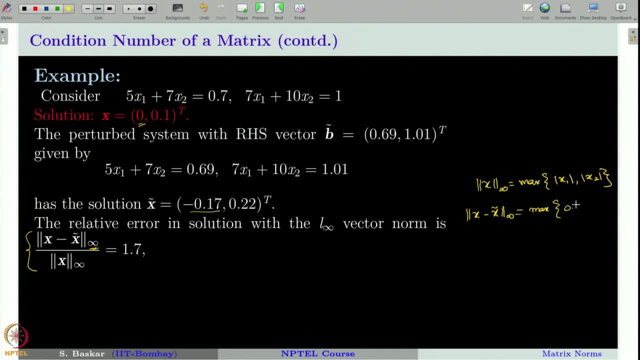 Therefore, its first component is 0.17, it is 1, 7, not 7, 5- and the second one is 0.1 minus 0.22, that will give us 0.12.. Therefore, this is 1.3 and 0.4.. Therefore, if you take norm, 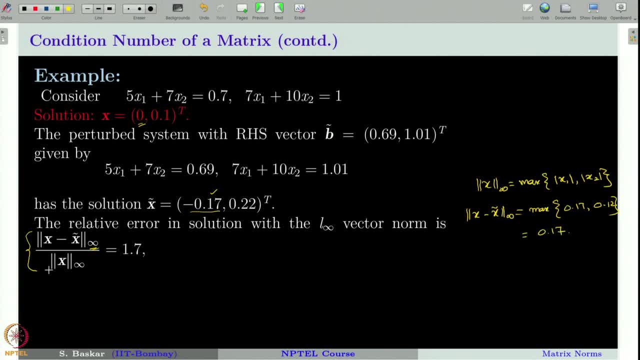 Similarly infinite norm of x, you can see that it is 0.1.. So the relative error in x tilde when compared to x is given by 1.7.. Now let us see what is the relative error in the right hand side vector. The right hand side vector relative error is 0.01.. Now you 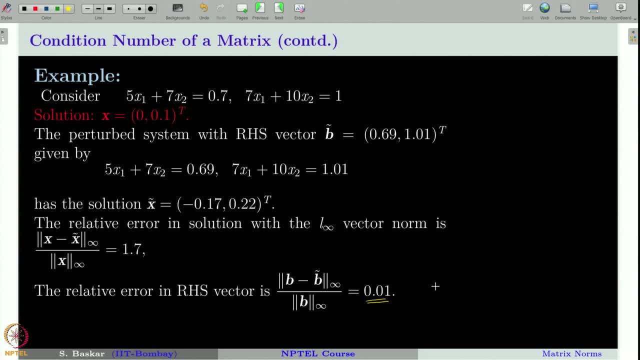 see in percentage, you have made only 1 percent error in the input data. that gave us 170 percent error in the solution. So that seems to be very bad. Now, the coefficient matrix in this system is very sensitive to the input data. Let us 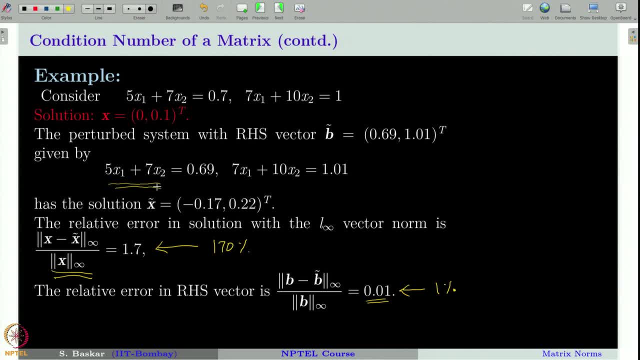 see what is the condition number of this coefficient matrix. The condition number of the coefficient matrix is 289.. How I computed this number? Well, I have taken the coefficient matrix as 5, 7,, 7, 10.. Now I have to find the subordinate matrix norm of A. What is that subordinate matrix? 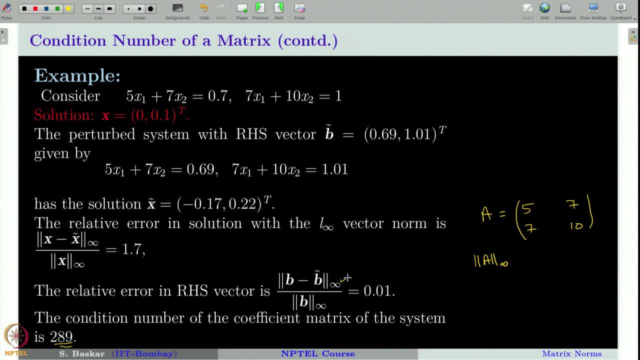 norm That is subordinate to the infinite norm. In the last class I have given the formula for this. So you go back to our previous lecture and get the formula for this and compute this, And also you find the inverse of this matrix and similarly you can find the subordinate. 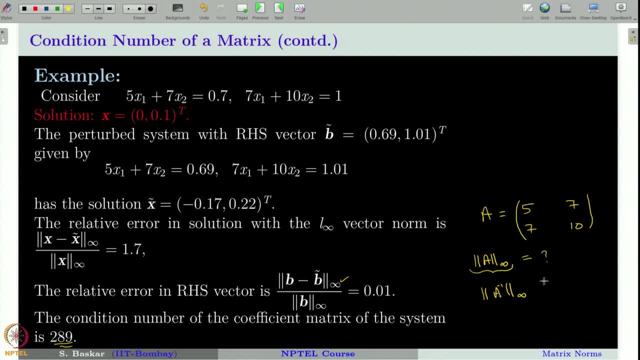 matrix, norm of the inverse of this matrix, and find this number also and then multiply both of them, because the condition number is nothing but norm A. Here we are taking infinite norm. Therefore you have to use that formula into A inverse- again infinite. 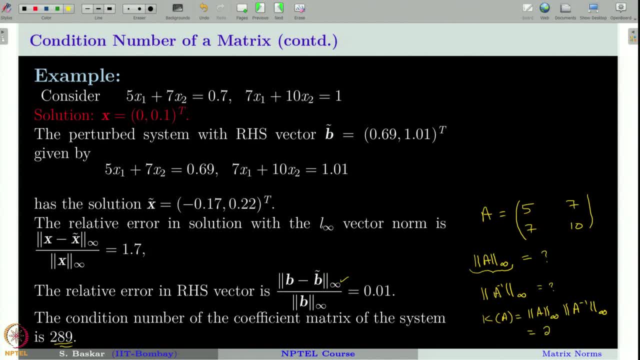 of A inverse, that will happen to be 289.. So you can see that the condition number of this matrix is pretty large- it is 289- and therefore, when you are working with a matrix whose condition number is very large, then you have to be very careful, because even if you make small, 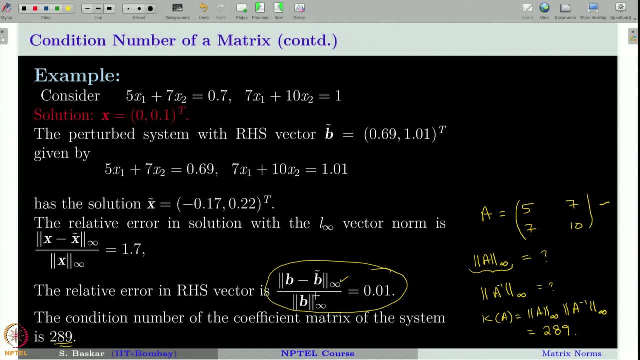 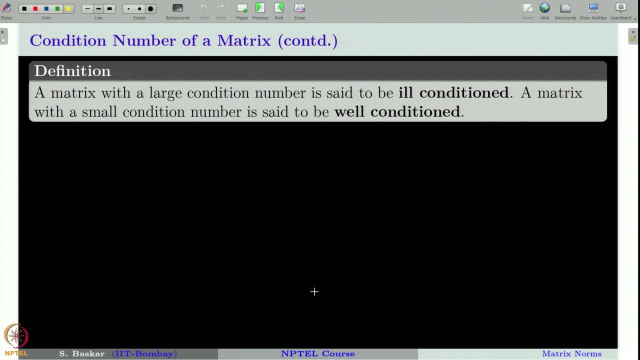 error in your input. here we made a error in the right hand side vector. Similarly, you may make a error in the coefficient matrix also. Accordingly, it will also magnify the relative error in the approximate solution. A matrix with a large condition number is: 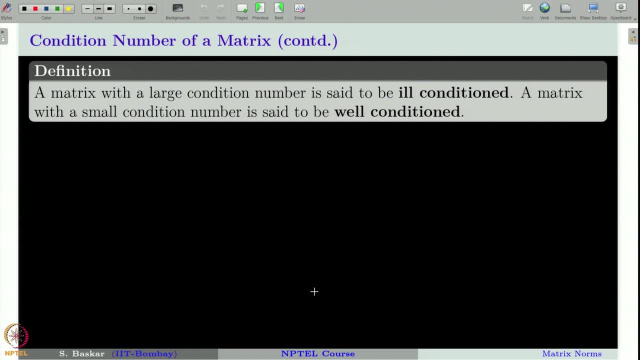 said to be ill-conditioned, whereas a matrix with small condition number is said to be well-conditioned. I have also introduced, in the case of evaluating a function, a C 1 function at some point in one of our previous classes, right. So here the words large and small is, in general, very 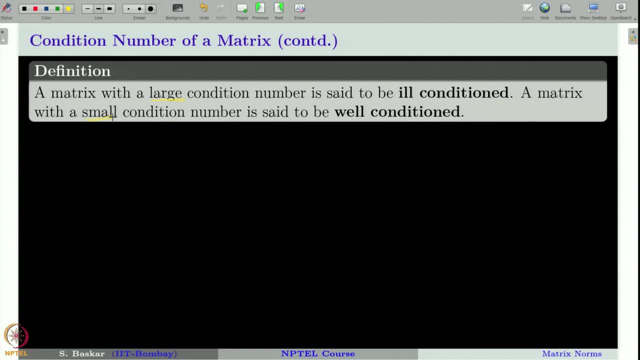 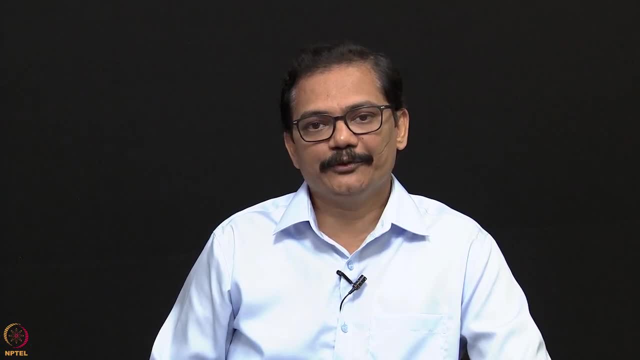 difficult for us to quantify how large it is and how small it is, because it depends on many factors. more importantly, it depends on the computational power. A more powerful computer can handle a very bad matrices relatively better than a small computer. Also, it depends. 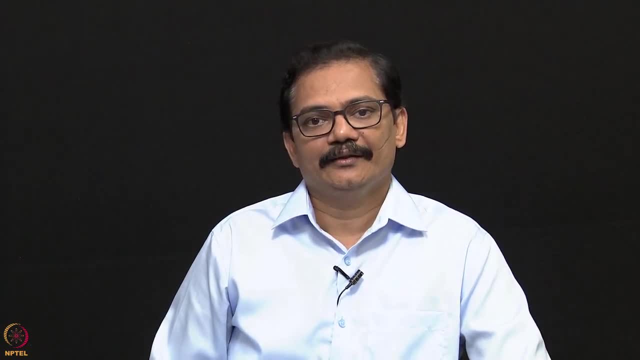 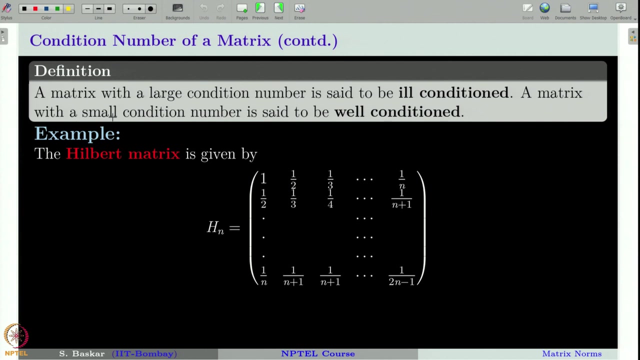 on what kind of applications that we are working in. Therefore, in general we cannot quantify what is large and what is small. Let us recall a very famous matrix called Hilbert matrix, which comes quite often in computers. In many mathematical models, just with n equal to 4, one can see that the condition 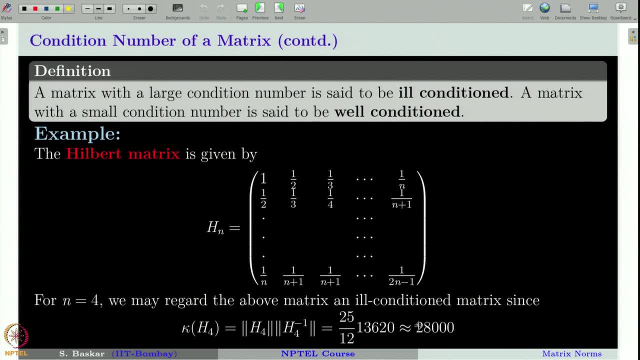 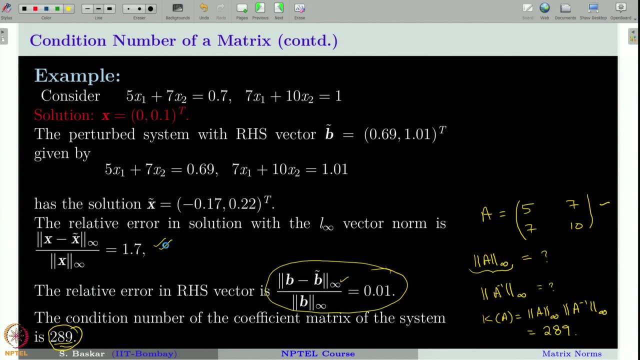 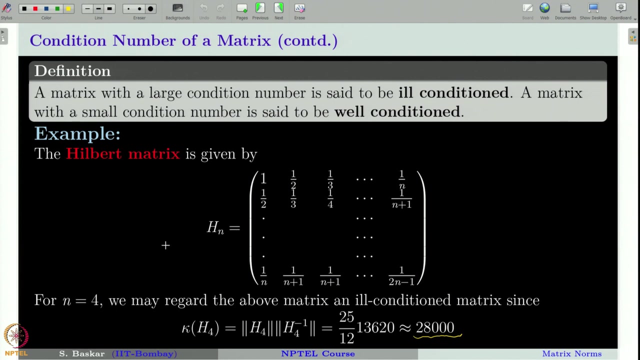 number of the Hilbert matrix H 4 is something like 28000.. Now you can imagine if a matrix of condition number is amplifying the error in the solution, so much what will happen to such matrices. This really tells us how serious it is for us to understand and then work with the matrices. 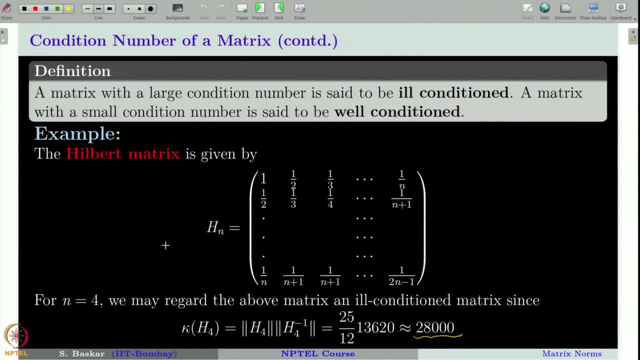 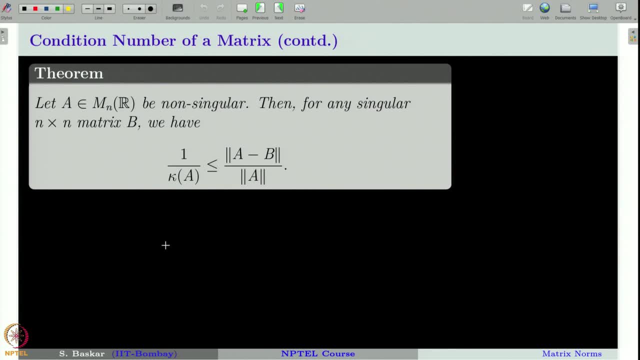 just going blindly with matrices and their computation is very dangerous on a computer. right Before ending this lecture, let us prove an important theorem which tells us how one can identify this matrix right Seeamos, and then works on this matrix a bad matrix, that is, a matrix with large condition number. Generally it may not be possible. 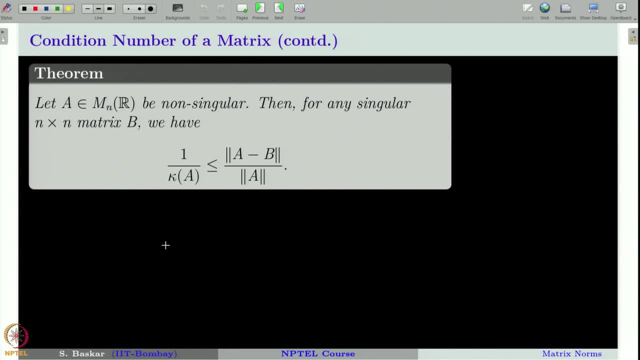 for us to use this theorem in practical situations. However, it is very interesting from the mathematical point of view. The theorem says that let us take a non-singular matrix A. then for any singular matrix B you have 1. by condition, number of A is less than or equal to the relative. 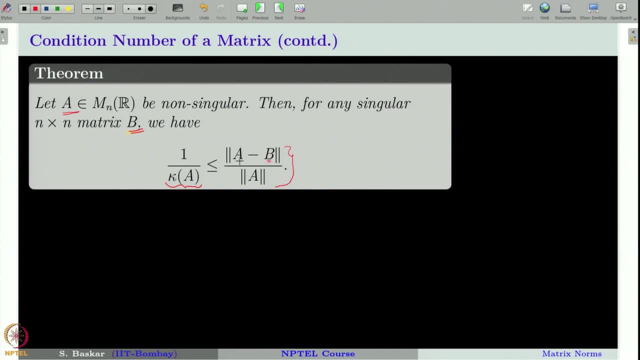 error in B when compared to A. Therefore, if A is very close to B, you can see that the relative error is going to be very small and that will make the reciprocal of the condition number to be very small. It means the condition number is very big. So this theorem says that if you are working, 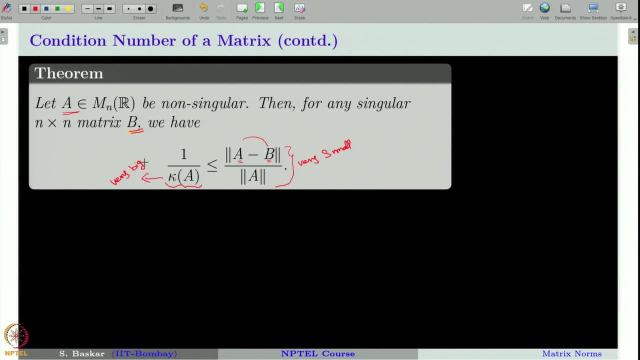 with a matrix which may be non-singular, but if it is very close to a singular matrix in this sense, then the condition number of your original non-singular matrix will be very large. That is what the theorem says. Let us quickly go through the proof of this theorem. 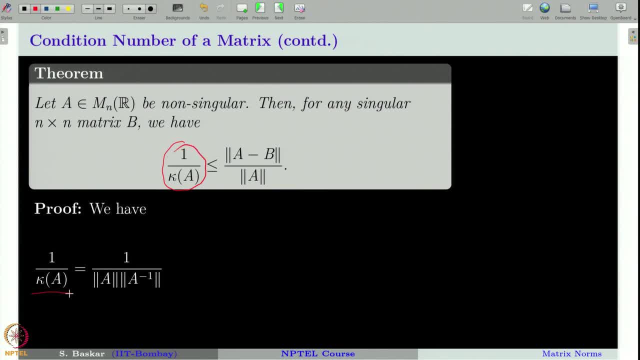 You take the left hand side 1 by kappa of A. I am just putting the definition of the condition number. Now I will fix this term and apply the subordinate matrix norm definition only for the second one, that is, norm A inverse. If you recall from our last lecture this: 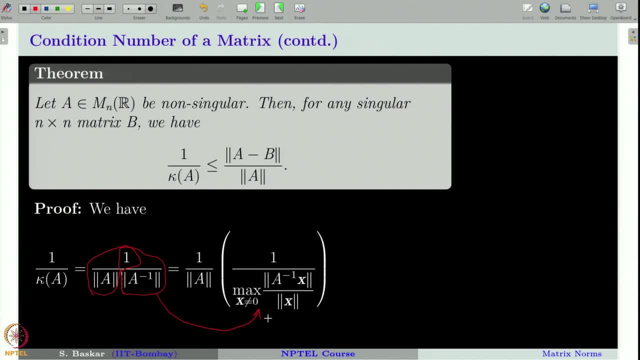 is a definition of the subordinate matrix norm. Now I will simply take this: instead of this maximum, I will take a arbitrary vector, y. Then what happens? I will just forget this maximum. Therefore, I will have less than or equal to remember, norm A. inverse y divided by norm y is less than or equal to maximum. 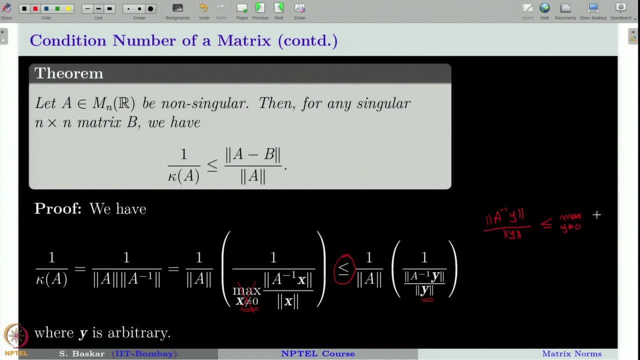 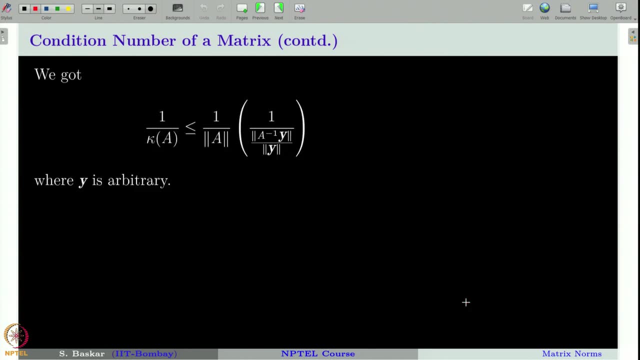 The value of this is the Oldman sum ok, of y to alpha than, or equal to Y by zero. Therefore, 1 by this will be 1 by this, but the inequality is reversed. That is what I have written here. We got this inequality for our condition number. let us 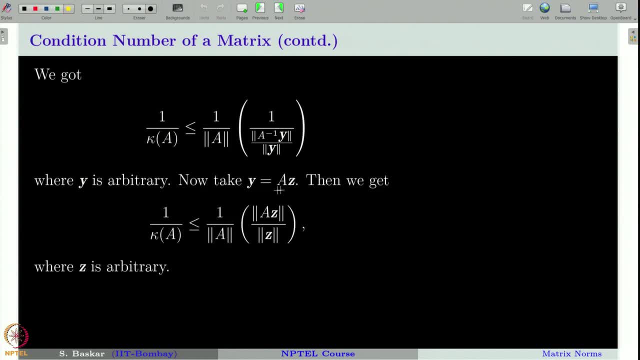 see how to go ahead with it. I will just put: y is equal to Az, just to make this term to look little better here. thereby I have 1 by norm a into. this goes to the numerator. I have a z divided by a inverse. y is now written as z, So this: 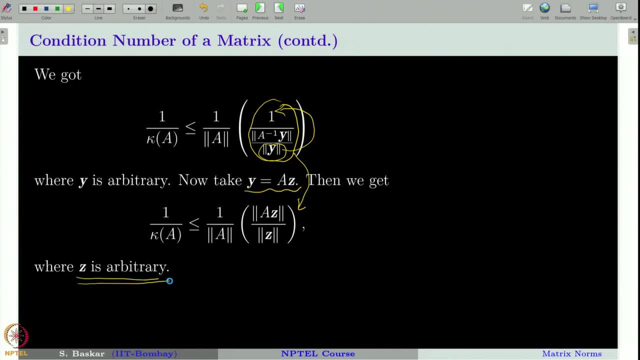 holds for any z. that is what we have seen. Now you take a non-zero z, such that b z equal to 0, how is that possible? Well, you go back to the theorem and see: b is a singular matrix. therefore this is possible. that is, you can find a non-zero vector z such that b z equal. 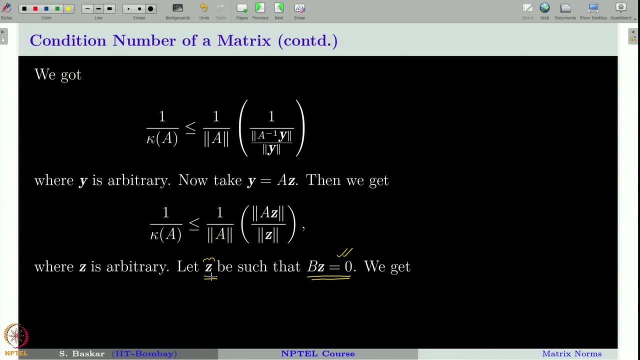 to 0.. Once you have such a z, remember this inequality holds for any z. I will in particular, take my z such that b z equal to 0. Therefore I can write this term as norm of a z minus b z. there is no harm in writing. 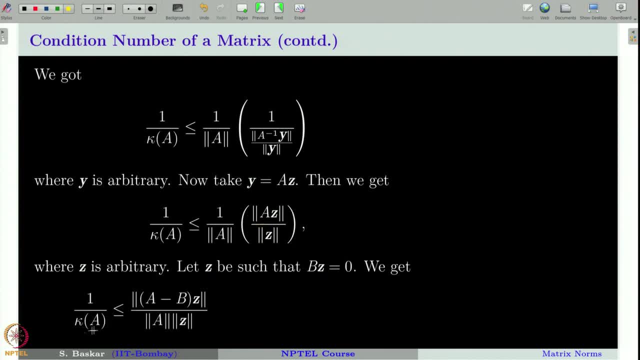 it because this is 0. So I will write: 1 by kappa of a is less than equal to a minus b z divided by this. this is there Now. I will use wherever you see norm a x kind of expression. you should immediately remember our property of the subordinate vector. 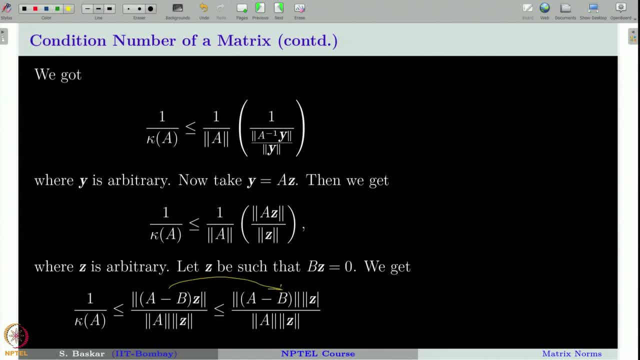 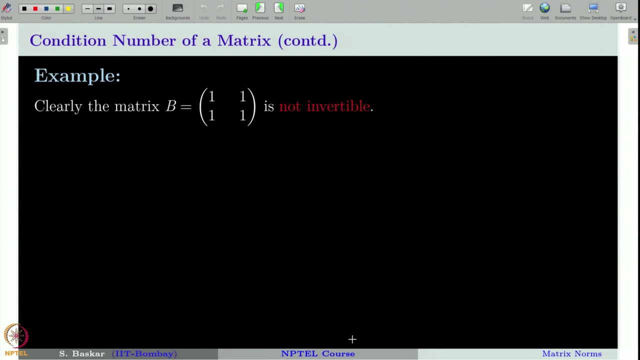 Subordinate matrix norm. you put that here. this is less than or equal to norm of a minus b into norm of z. Now z gets cancelled and you got what you want, and this is what the theorem says. Let us see quickly an example for this. let us take the matrix b, which is: 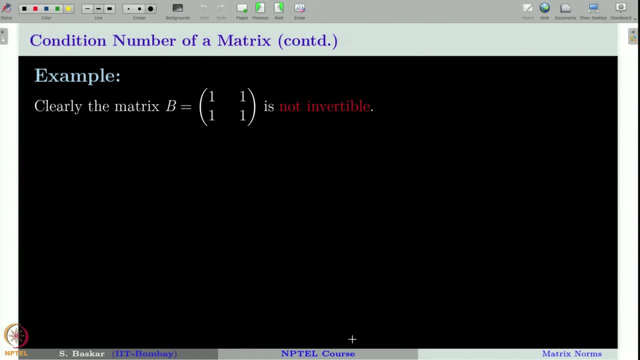 equal to 1, 1 1 1, which is not an invertible matrix. Now let us perturb the matrix b little bit by adding epsilon to some of its terms and call this as a. As long as epsilon is greater than 0, this is a non-singular matrix. Therefore, 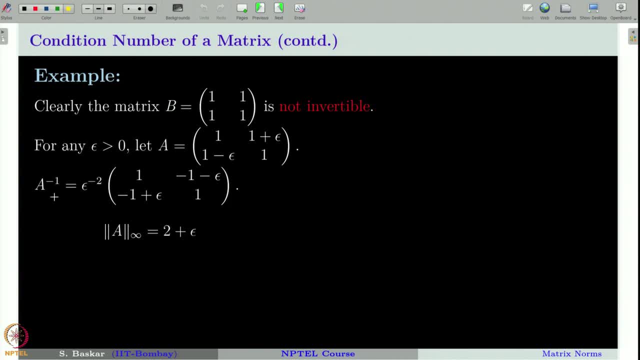 you can find a inverse for this. and now, what is norm a with respect to the subordinate matrix? norm to L infinity norm, Since it is like this quantity. you just go back to our previous lecture. recall what is the formula for this. come back and apply it to this matrix. you will get this inside. 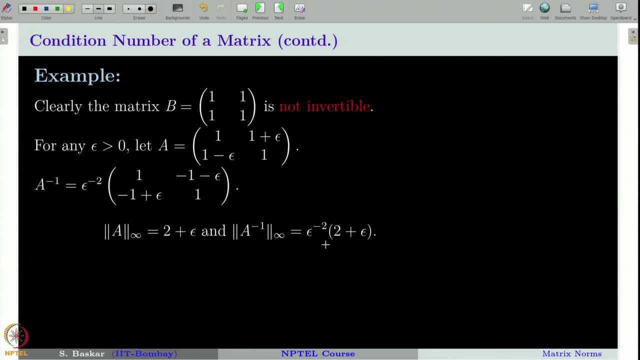 and similarly norm a inverse is given by this. Therefore, the condition number of the matrix a is given like this, which in our case is given by this expression, and that can be greater than 4 by L infinity epsilon square. Now you see, if you take epsilon very small, you can see that the condition 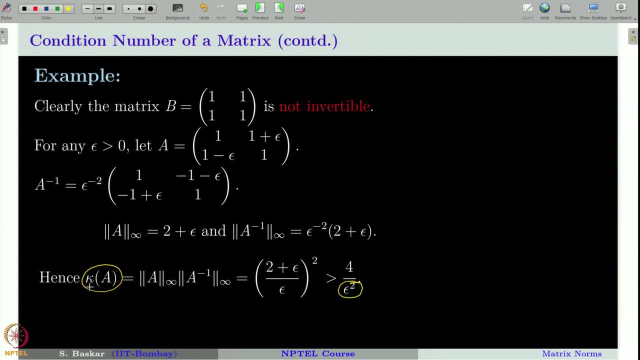 number of the matrix A is going to be very large, right? So that is what is given in the previous theorem. also, we are just cross checking the theorem that we have proved just now in this example. just to be more precise, let us take epsilon to be something like 0.01. 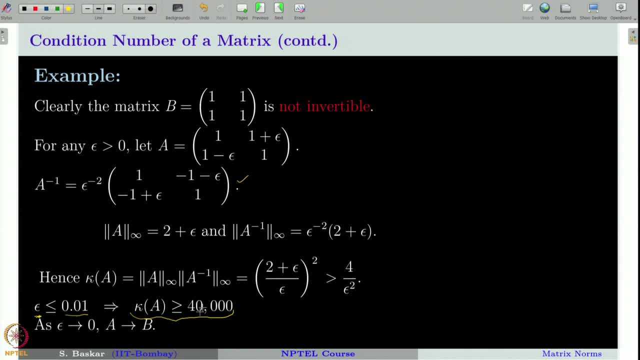 and that leads to your condition. number of the matrix A has something like 40000.. You can also see that your matrix A is pretty close to the singular matrix B whenever epsilon is very small. that is what is written here And consequently, if you just take epsilon, 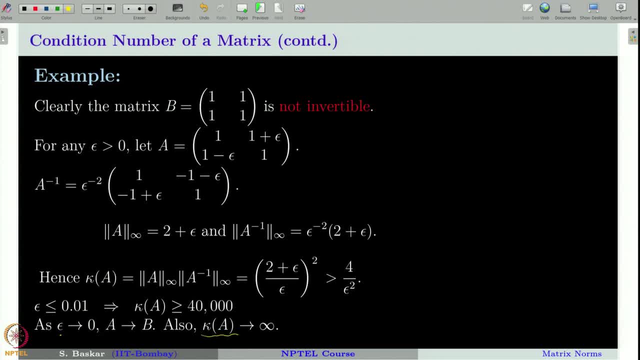 going to 0, you can see that the condition number of A will in fact tend to be very small to infinity right. So this tells us that if you are working with a matrix which is very close to singular matrix in the sense that is defined in the previous theorem, then 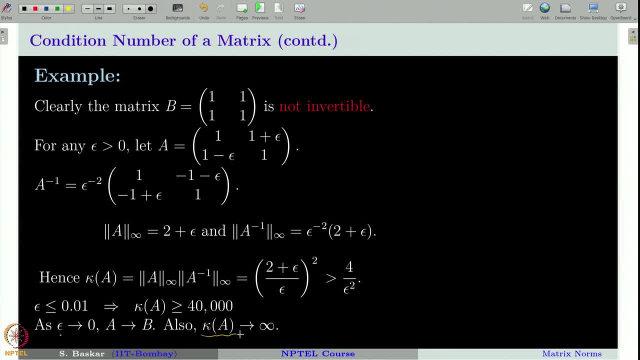 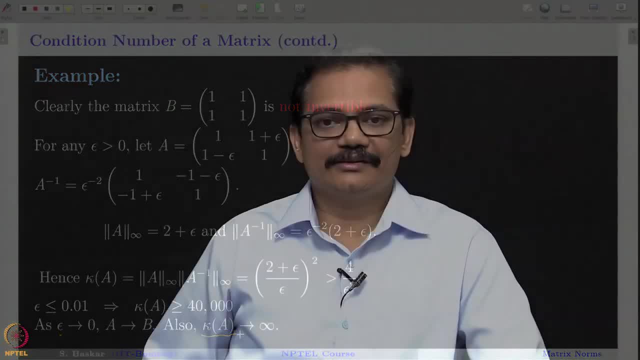 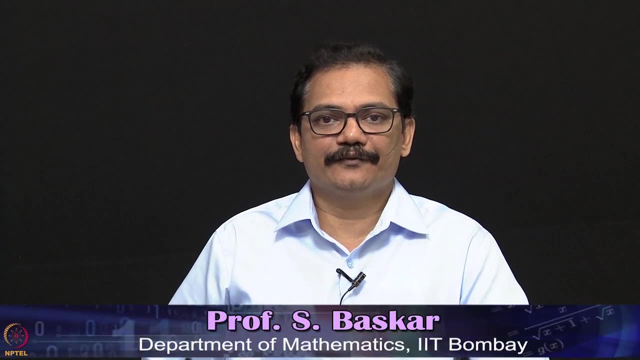 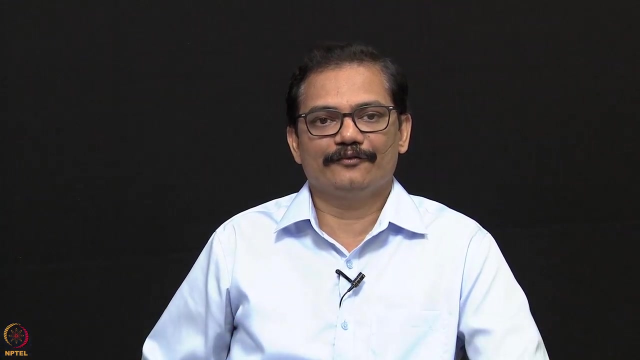 you are likely to have very sensitive computation for your input data. So in this lecture we have understood what is mean by condition number of a matrix and how to learn the sensitivity of the matrix in computing solution of a linear system in terms of condition number of a matrix. 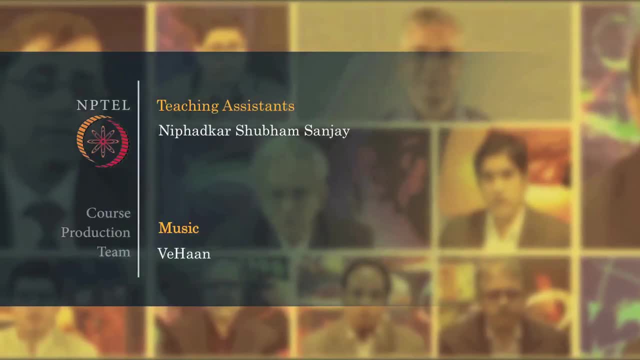 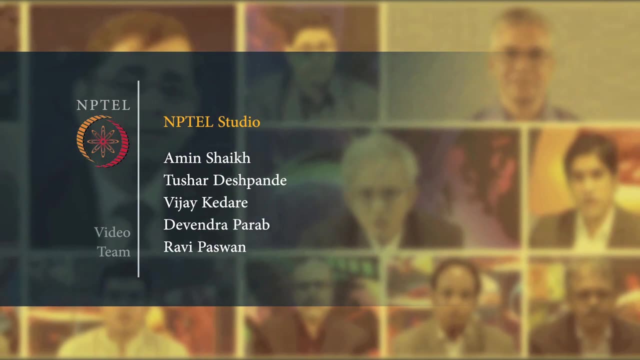 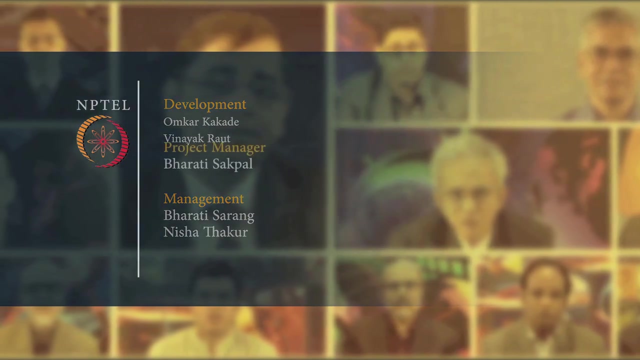 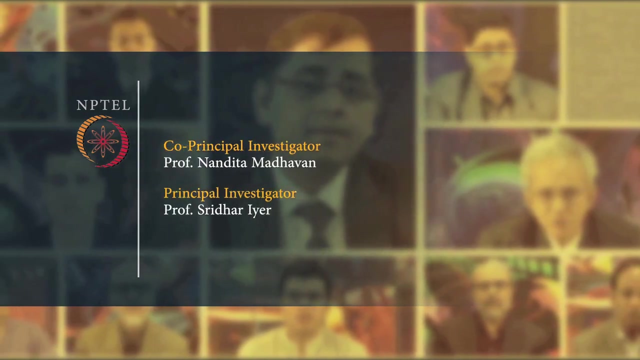 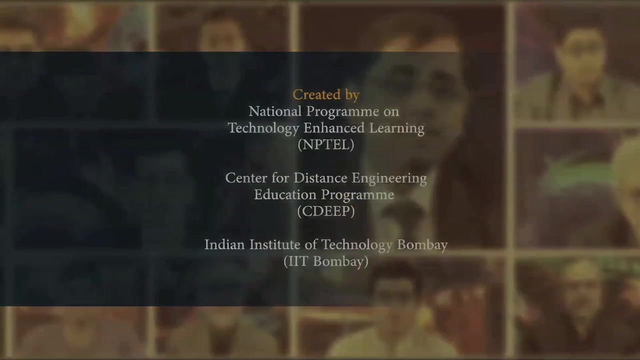 Thanks for your attention, you.